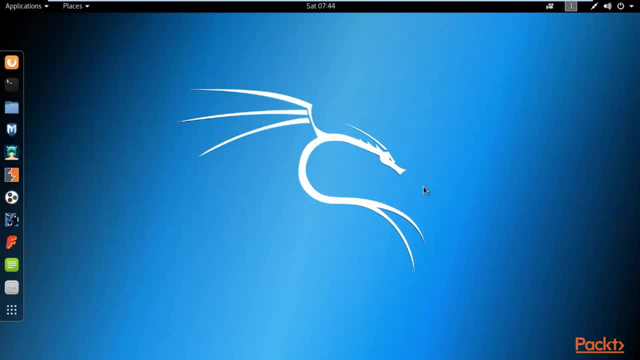 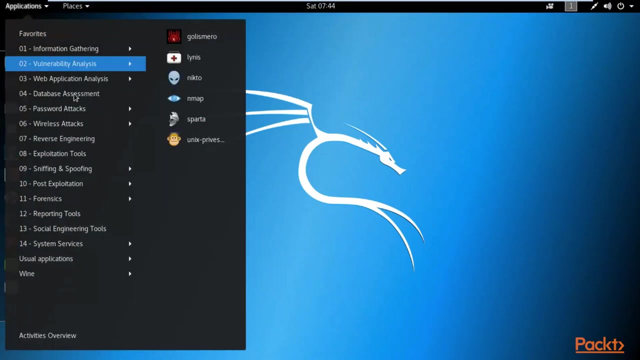 So, guys, here we are at Kali Linux operating system and first of all I will show you that how to perform MITM using wireshark tool. So here you can see the lab. I have Kali Linux open and Windows open right, and so click on applications and you can select sniffing and spoofing, and here you will find the wireshark inside it. So click on it and open it and this is the Windows machine. This is our Windows machine. 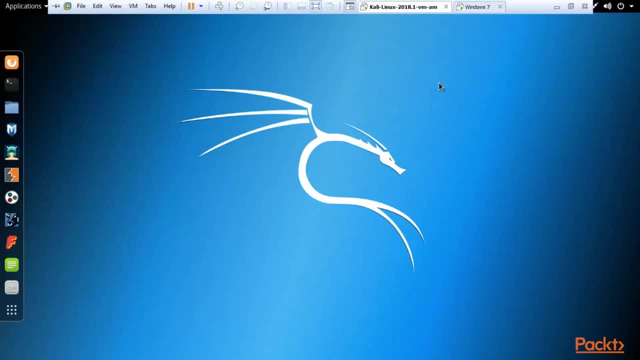 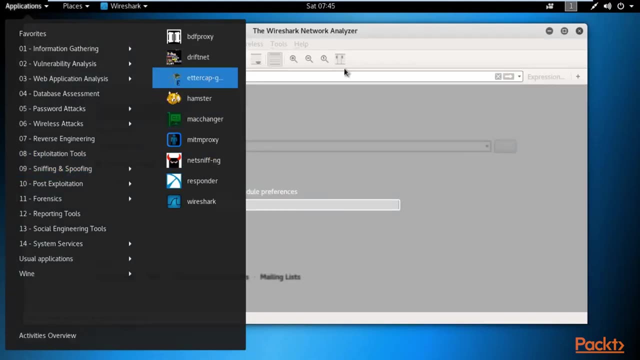 This is our victim machine and Kali Linux is our attacker machine. Intercap is also available there. You can see here. intercap is also available, Here it is, So we will perform it. First of all, we need to take a look at wireshark. 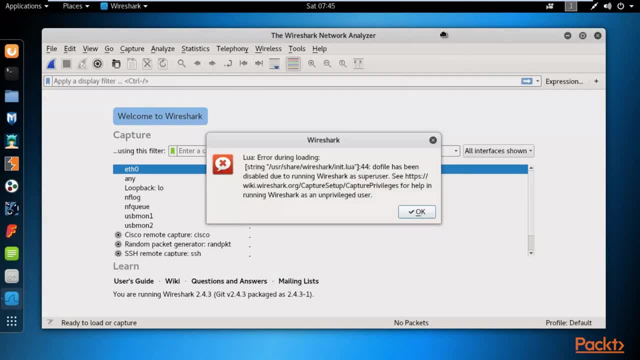 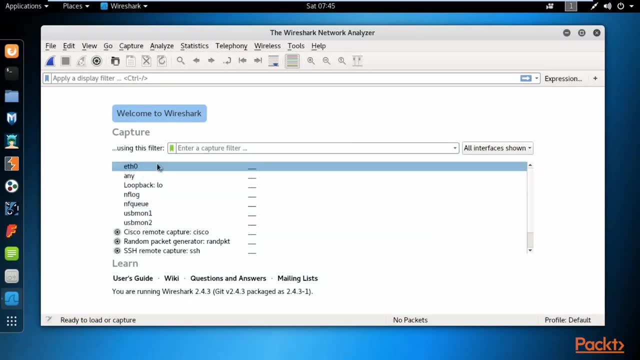 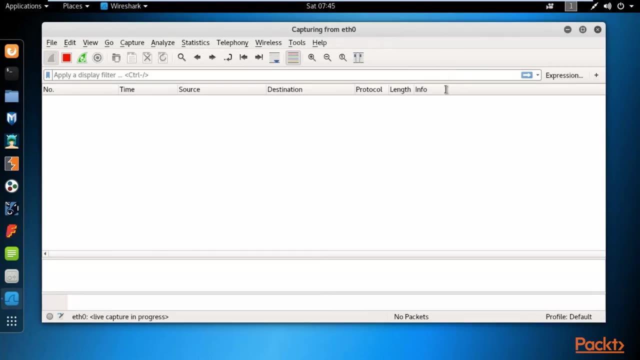 So this is wireshark network analyzer. Here you need to select. first of all, this is a list of adapters you need to select. Here we are working on Ethernet 0. So double click on it and open it. Now you need to go back to Windows. 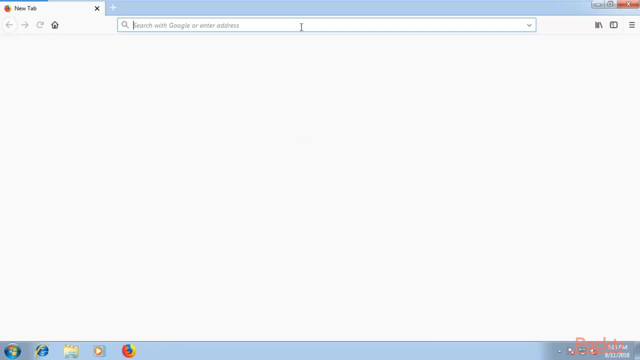 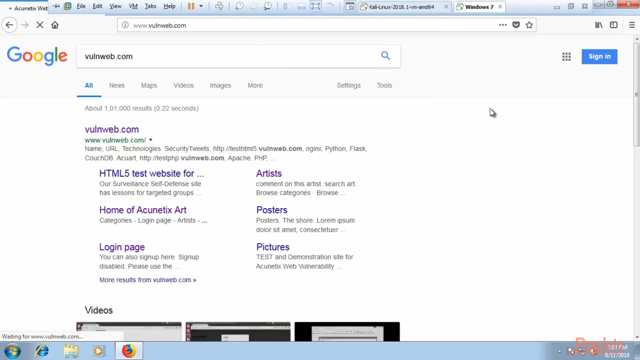 Open the browser, Open googlecom. So here, Google has been opened and you need to open the website. For example, let me just open the login page of any sample waitsite. This is the sample website. Open the website And click on the second link. 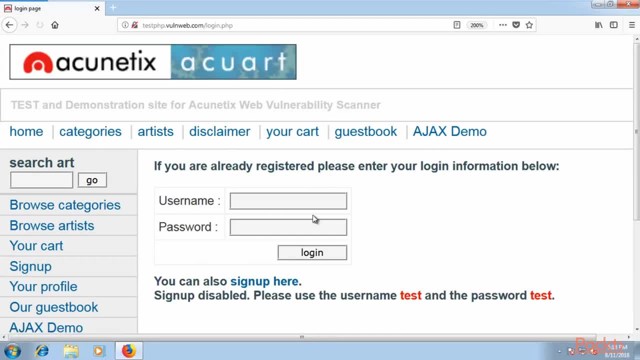 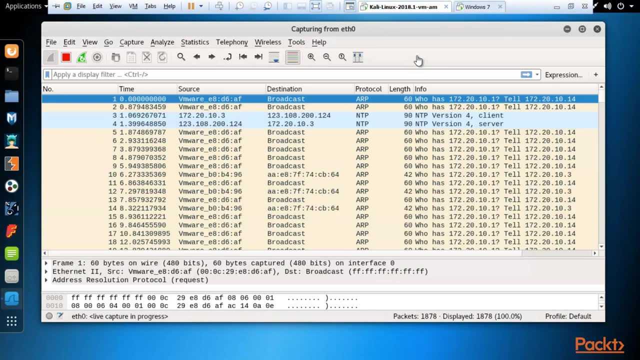 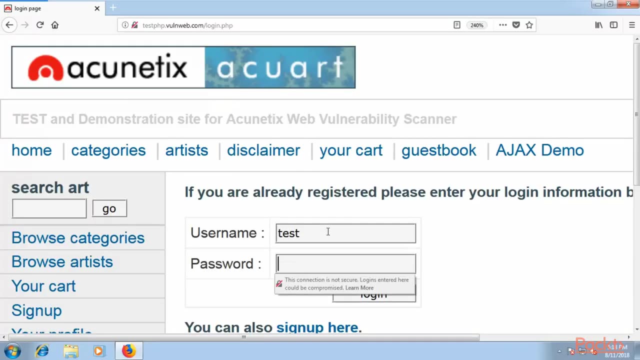 Then click on sign up. So, for example, the victim is trying to insert, For example, is login and password and username and the password block, right? so how wireshark can capture that data that I'm going to show you. so do one thing: type here something as a victim. for example, the username is test and the password is. 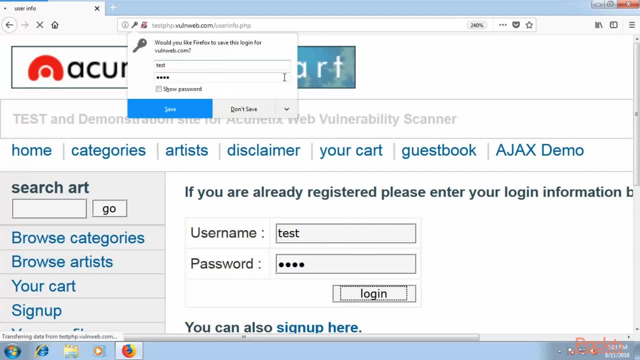 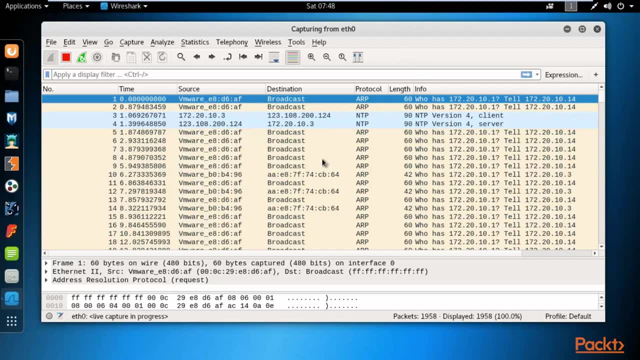 also test all right, click login, right. okay, now go back to Kali Linux operating system and I hope the wireshark has already captured the login credentials. so I need to stop sniffing process. right, so you can click on this red button to stop sniffing. so let me click on it right now. we need to select that. 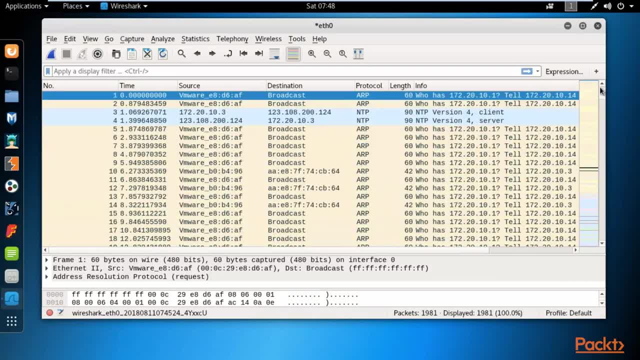 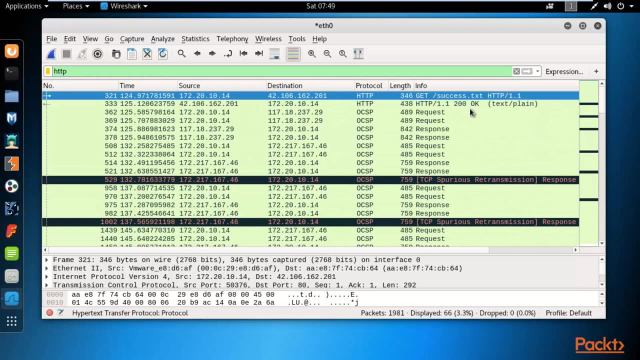 which packet contains the username and the password. so we need to use a filter to find out. so, for example, in filter you can type HTTP and hit enter, because we were using HTTP website and here still there are so many HTTP packets are available, so we need to find out which. 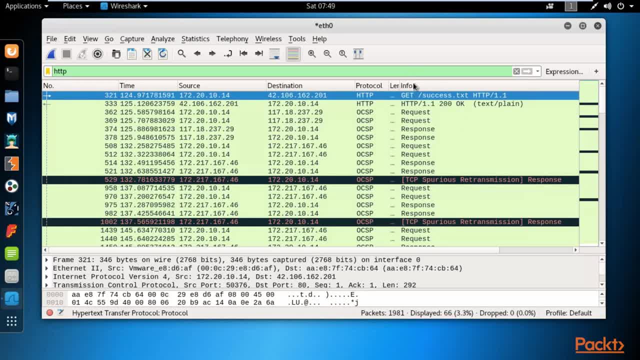 one is useful for us. so we need to you select the info part and inside info part. you need to find out that which one is useful. so I am. I'm basically choosing the packets which are using post method, right, so I need to select where is the? 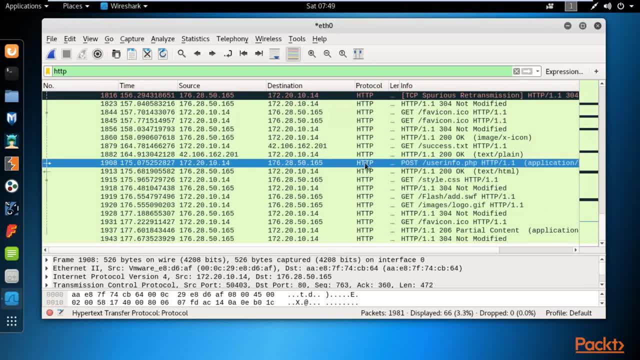 post method. here I can find out this packet using the post method and it is written inside the info part. so this is the source. source is basically the Windows machine. I used to use Windows machine. I used to use Windows machine, I used to use Windows machine and this is the text input of our chip. I am going to 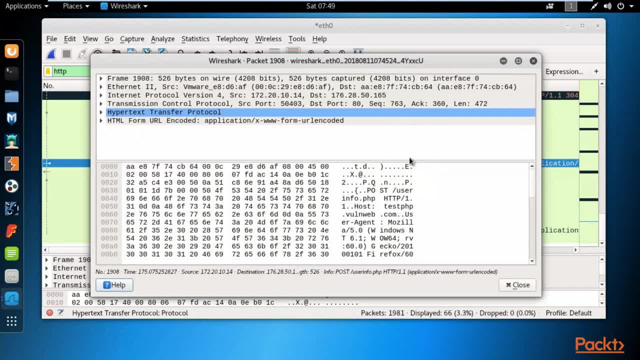 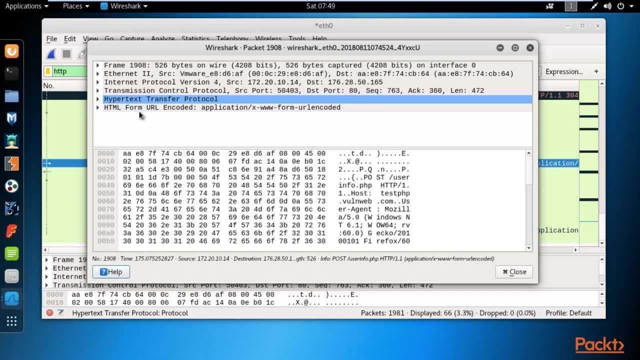 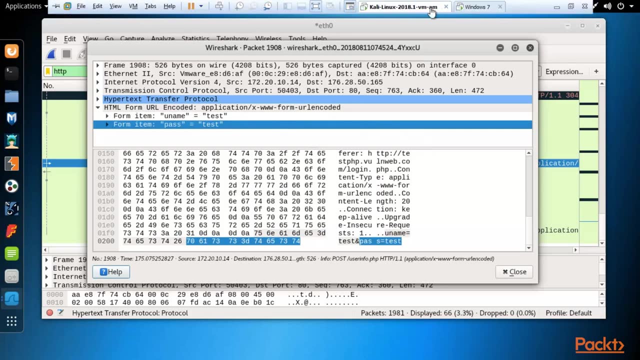 search for the IP address destination and this will be IP address of the server of the website. so double-click on it and here we need to find out where is the username and the password. so here you can see it is written HTML form URL encoder when you will click on this, so you can see here that username test and 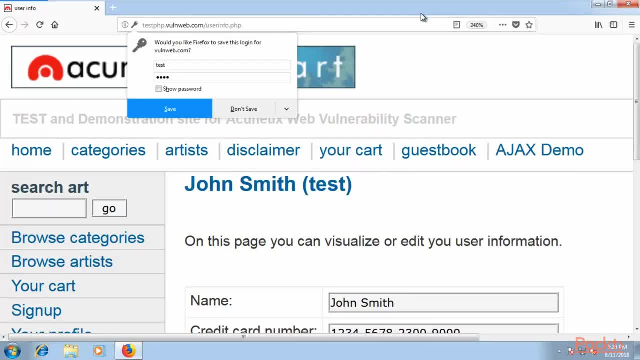 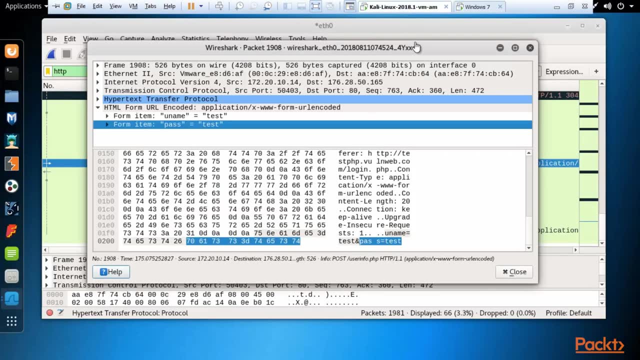 the password test has been captured using wireshark. it means what have a username and the password you are using inside Windows machine. it has been operating system. so this is a simple example of man-in-the-middle attack when the operating system is trying to connect with the web server. so in the 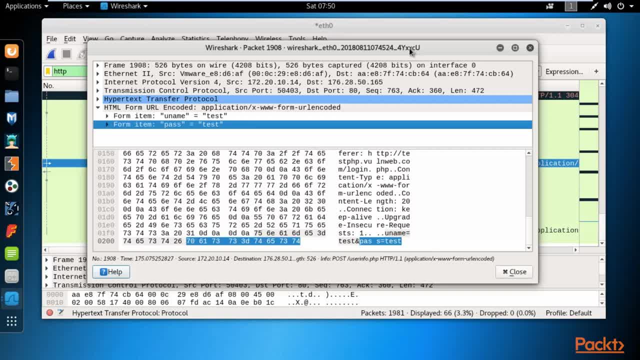 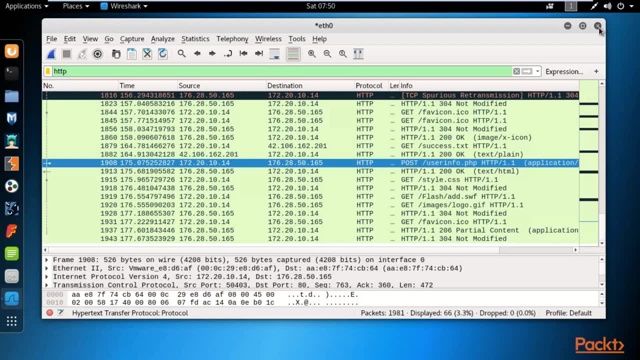 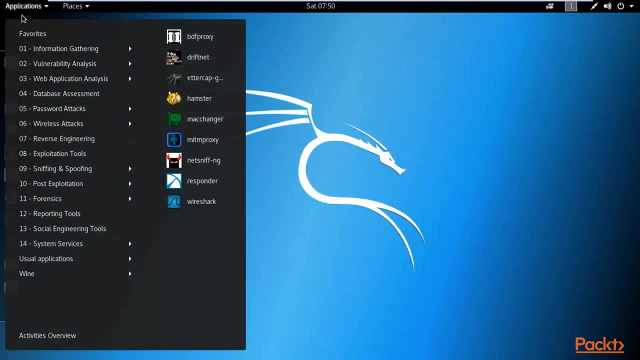 middle Kali Linux operating system is trying to sniff the data, and they have successfully done it. so this is basically: MITM is using wireshark software. now I am going to show you another tool, which is ATA cap. so click on applications, select sniffing and spoofing, and then you can click on ATA. 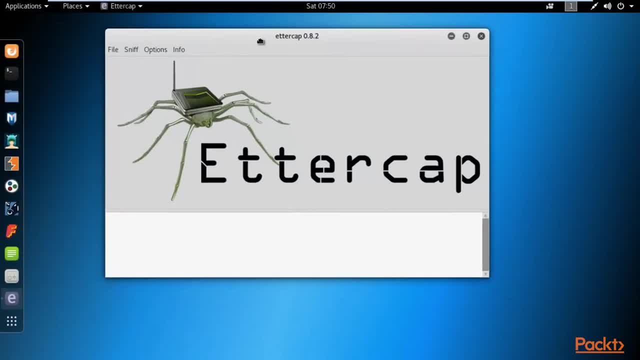 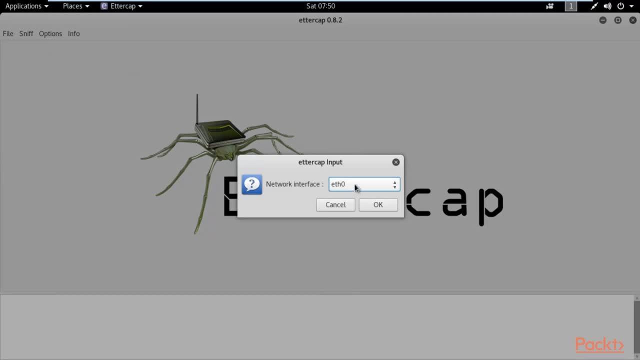 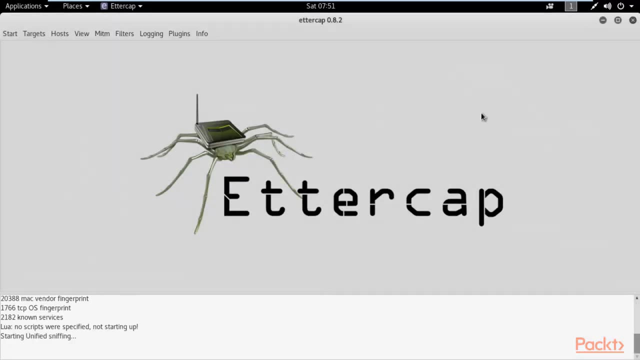 cap. so this is ATA cap, right? do one thing first of all, click on sniff data, select unified sniffing. you need to select your interface here, which adapter. so I'm using eth0 to select eth0. click OK. unified sniffing is starting. now I need to check that. how many machines are there in my network? so I need to click. 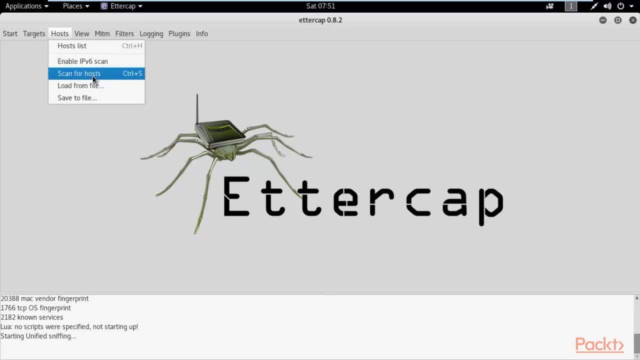 on hosts, click on host list or you can scan for hosts. so let me click on scan for hosts, so it is showing that four hosts are added. so let me check the IP address. so click on host, select host list, and here are the IP address. so this is will be. 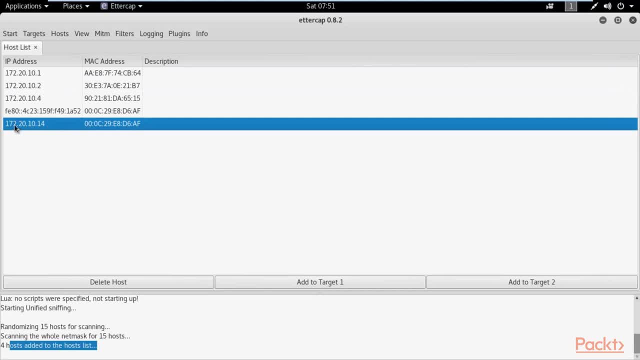 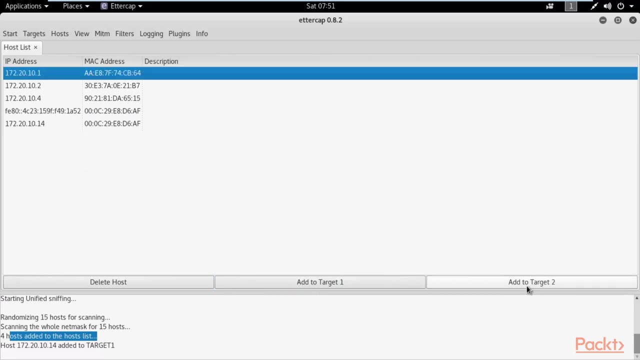 your gateway, right. and these are other machines. and this is the IP address of Windows operating system, right? so first of all select the victim machine IP address. click on add to target one. added the target one. now select the gateway, which is dot one. click to add to target to both have been. 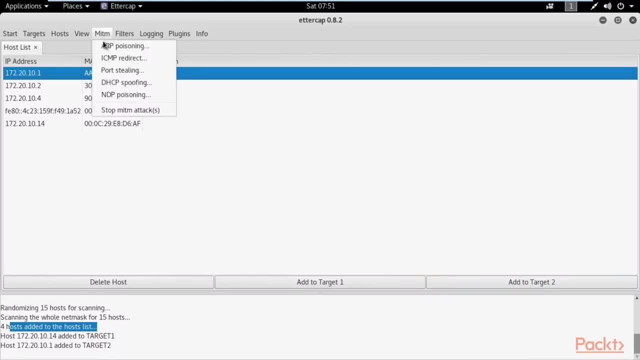 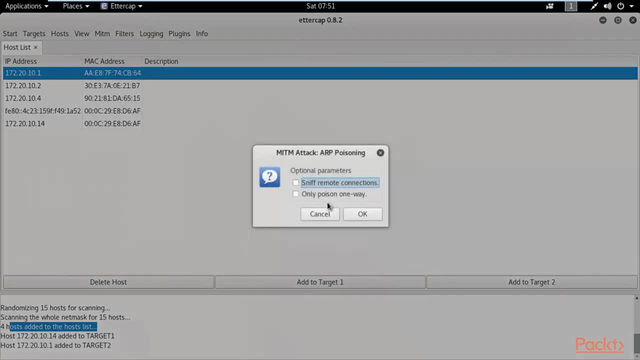 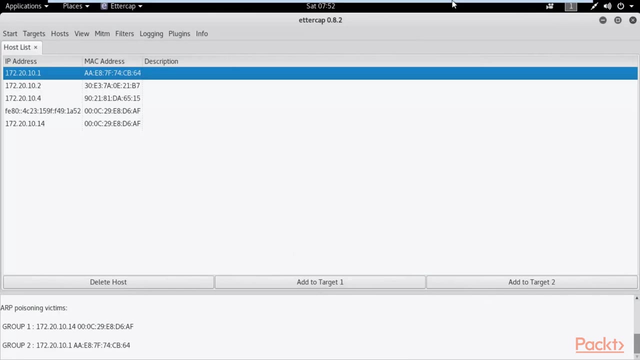 added. right now you need to click on MITM and click on ARP spoofing address resolution protocol- poisoning- right click on this and you can select on sniff remote connections. click OK and this is the setup. so now what? go back to the Windows machine. right, and let me go through the windows machine. right and let 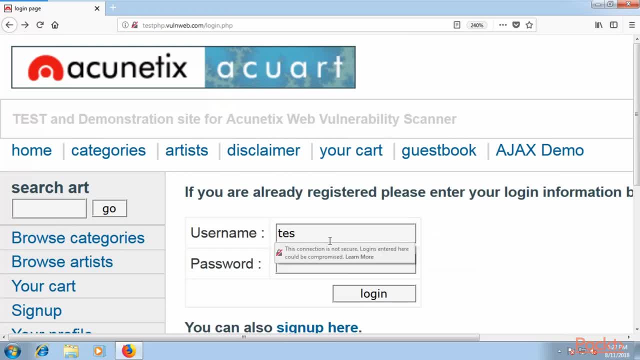 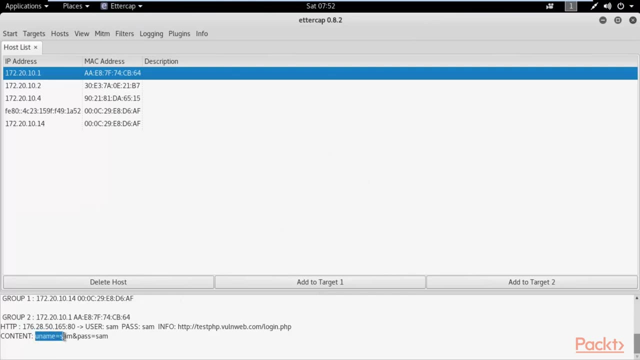 me go back to the username in the password panel and here you need, you can type any username in the password. for example, Sam is the username and Sam is the password. alright, click login. and when you go back to the Kali Linux operating system so you can see here that your username and the password has. 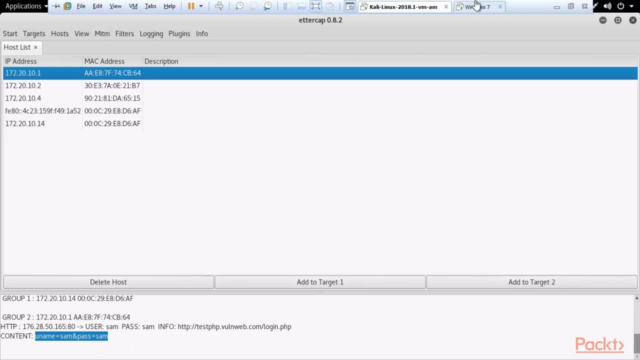 been captured by it, a gap inside Kali Linux. so basically we were in the same network. Windows 7 and win and the Kali Linux were in the same network, right? that's why in this case, that it can perform ARP poisoning in the network and by using our poisoning attacker machine can capture data from the victim machine. 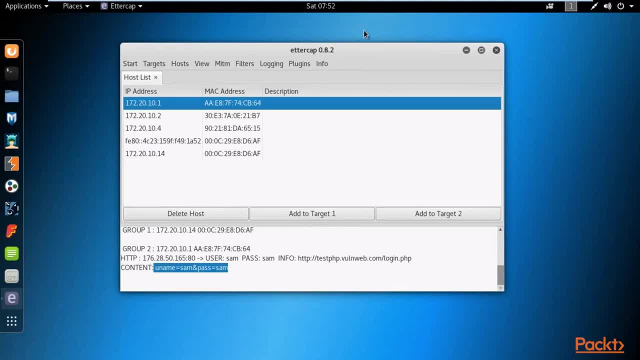 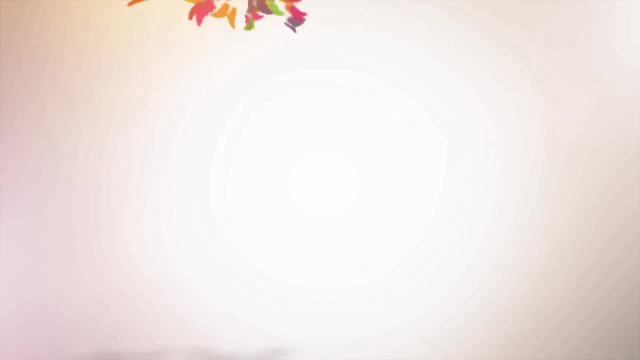 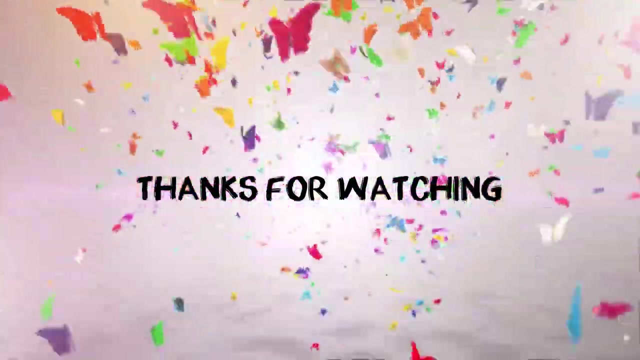 so this is a simple example of wire shock and a decaf that how these tools can capture these kind of sensitive information from the victim machine. so this is all about the man in the middle attack. I hope you have learned anything from this video. if you have any questions, please feel free to ask in the 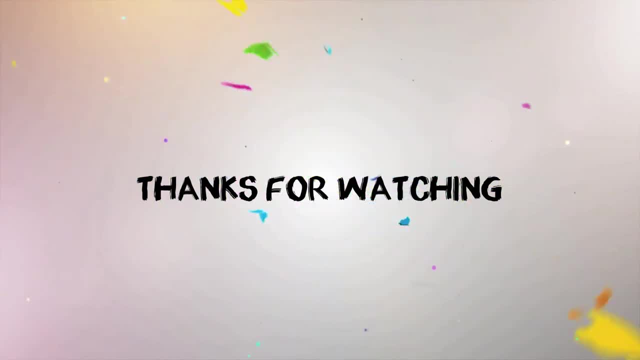 comments and I will see you in the next video. thank you so much for watching and I will see you in the next video. bye, bye.